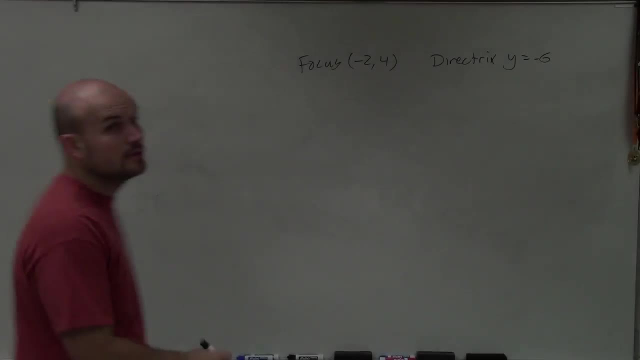 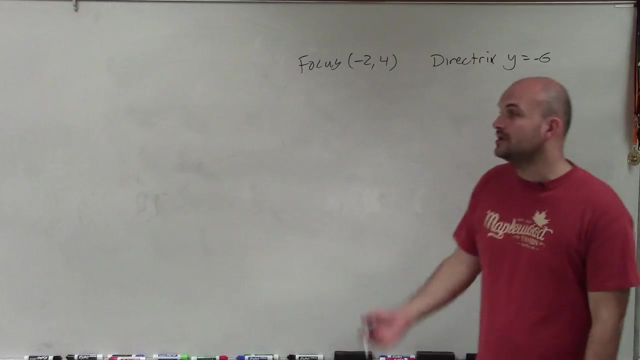 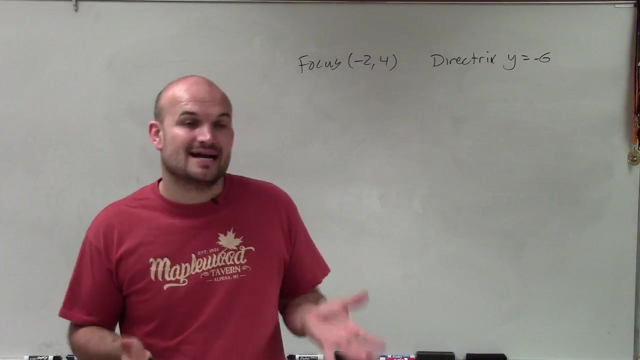 Welcome. So what I like to do is go ahead and go through writing the equation of this parabola, knowing that I have a focus of negative 2, comma 4 and a directrix of y equals 6.. So the first thing I need to do is identify: is my axis symmetry going to be vertical or 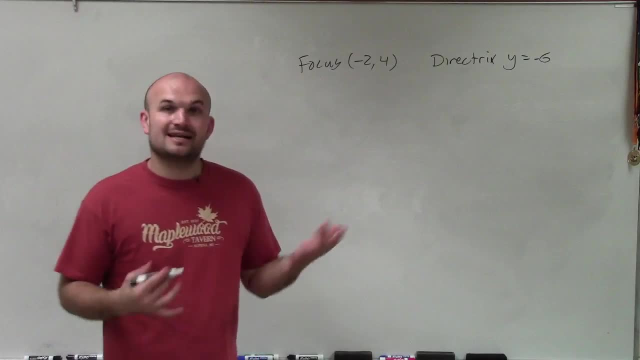 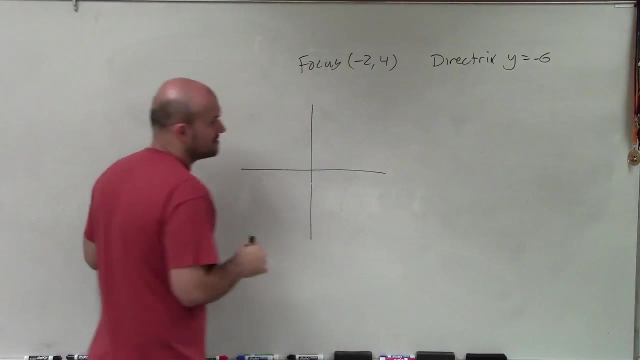 horizontal, And the only way I can be able to identify that is by plotting the information that I have, And once I know if it is vertical or horizontal, then I can determine what exactly is going to be what type of equation I'm going to use. So the focus at negative 2,. 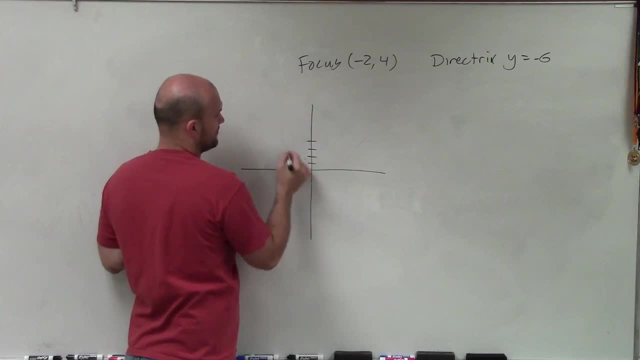 4.. So I go negative 2, up 4,, 1,, 2,, 3,, 4.. And my directrix is at negative 6, 1,, 2,, 3,, 4,, 5, 6.. Directrix is y equals negative 6 from my origin, which would be 1,, 2,, 3,, 4,, 5,, 6.. 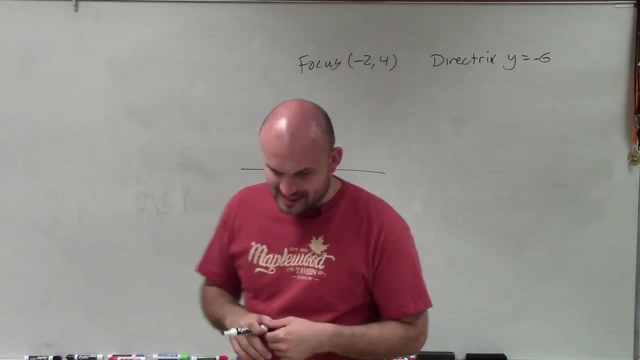 Okay, So now, in this case, what I'd like to be able to do is I'm going to go ahead and go through writing the equation of this parabola, knowing that I have a focus of negative 2, comma 4.. So the first thing I'm going to do is notice that. 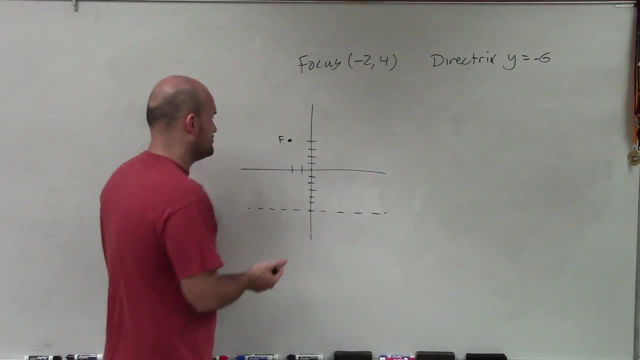 the distance between my directrix and my focus is going to be my vertex And remember, the vertex is always going to be opening towards your focus. So my parabola is going to open something like this: I don't know where the vertex is, but I'll figure that out in just 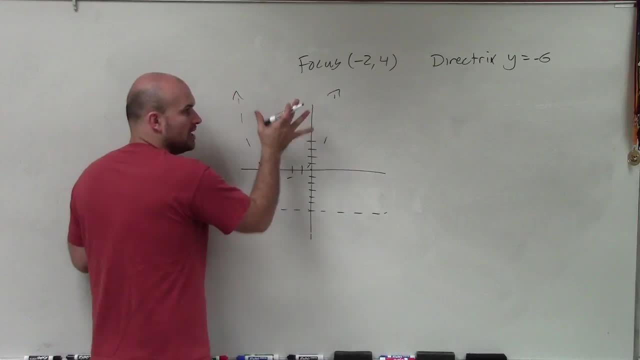 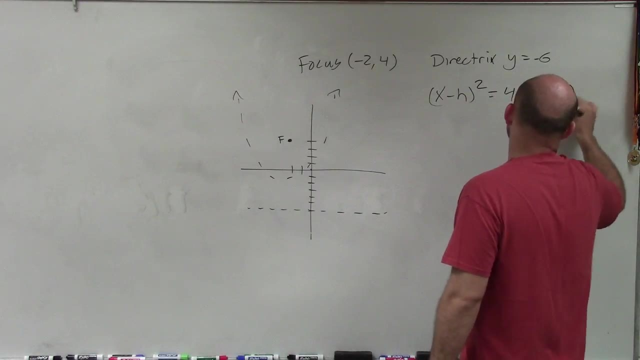 a second. The main important thing is: I understand that the parabola is going to open up. Therefore, that's going to tell me I can use the equation x minus h squared equals 4p times y minus k squared, or y minus k. Therefore, once I know that I have a focus of negative 2 comma. 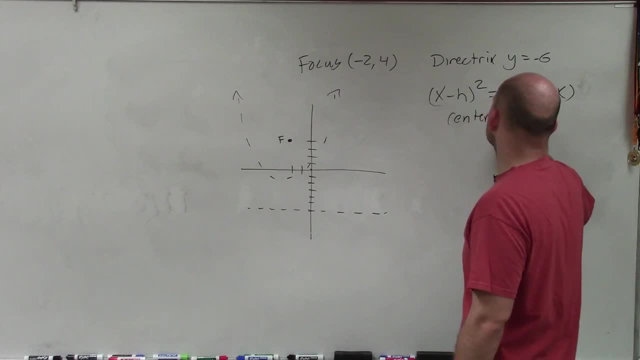 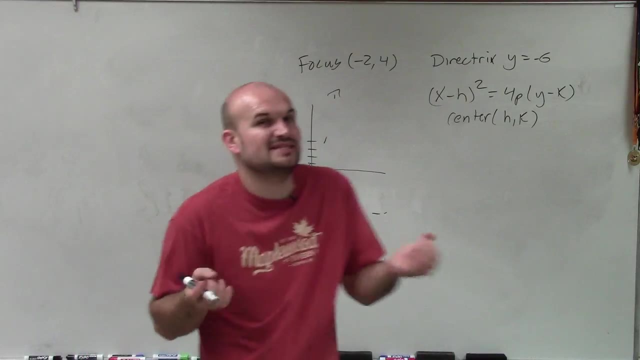 4,. once I know this and I figure out the center, that is going to be my points h and k. So let's go ahead and determine, because between the focus and the directrix- remember, the definition of parabola is that all the points on the parabola are equidistant from 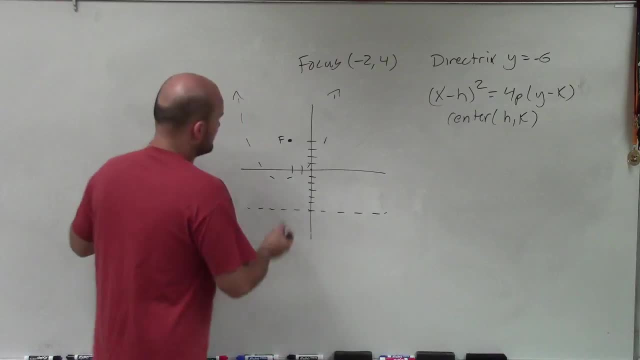 the focus to the directrix, including the vertex. But what's important is the vertex is on the axis of symmetry with your focus, which is perpendicular to my axis of symmetry. So if this goes up, 4. All right, And this one goes down, 6.. I can probably say that to find the midpoint between